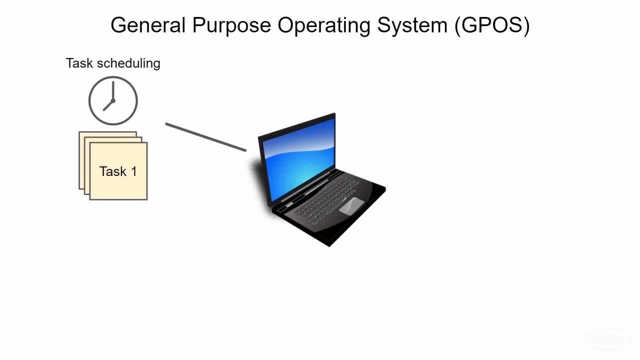 so that everything appears to be happening concurrently. Second, it manages a number of virtual resources like files, libraries and folders, allowing applications and processes to access them when needed. Third, they can manage or provide device drivers for your system. These drivers allow the system to read and write from an external disk. respond: 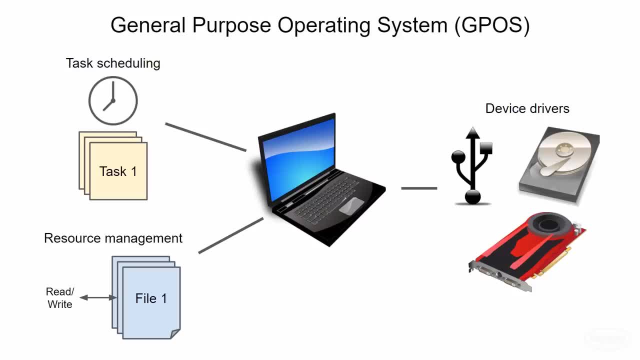 to keyboard and mouse input or draw graphics on your monitor. You're probably familiar with general-purpose operating systems like Windows, macOS and Linux. iOS and Android also fall into this category. Most general-purpose operating systems are designed with human interaction as the most. 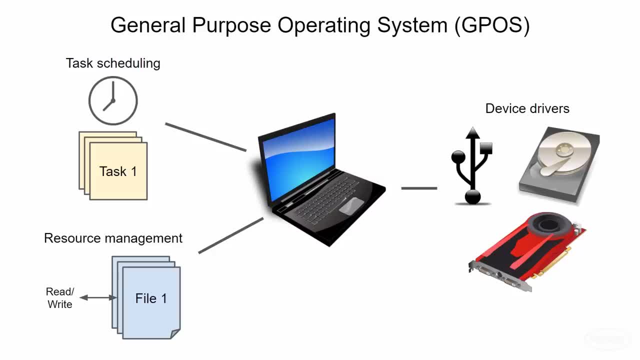 important feature, so the scheduler is designed to prioritize such tasks. That may mean some timing deadlines can be missed or pushed back, and a little lag in responsiveness- especially if it's not really noticed by a human- is acceptable. Additionally, the scheduler is often non-deterministic, which means we can't know exactly which task. 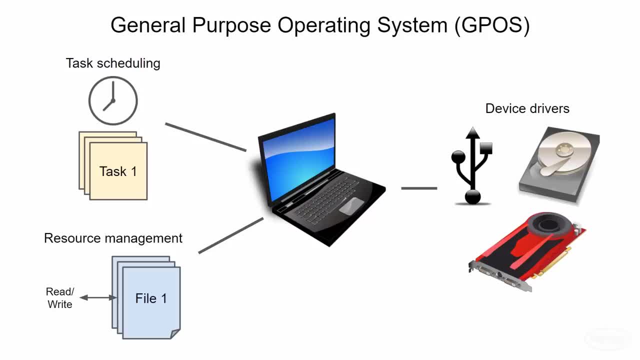 will execute when and for how long. If you're making something that requires an OS and strict timing deadlines, like a medical device or engine controller, missing a deadline to say, fire a spark plug would be catastrophic. This is where a real-time operating system, or RTOS, can save the day. 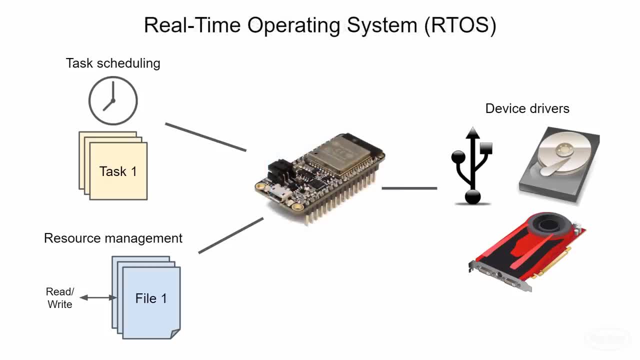 Most RTOSes offer many of the same functions as general-purpose operating systems, but they are designed so that the scheduler can guarantee meeting timing deadlines on the tasks. While some RTOSes might provide high-level device drivers, you'll usually see things intended for microcontrollers like Wi-Fi and Bluetooth stacks or simple LCD drivers. 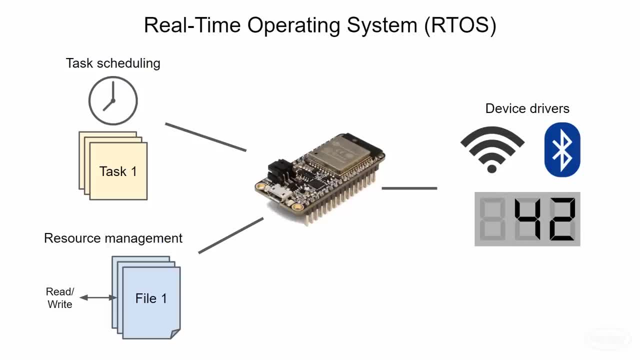 You can also find bare-bones RTOSes that provide just a scheduler. With these, you'll need to import or write your own schedule. You can also find bare-bones RTOSes that provide just a scheduler. With these, you'll need to import or write your own schedule. 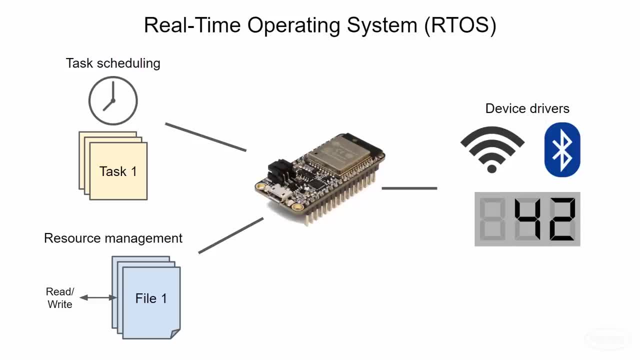 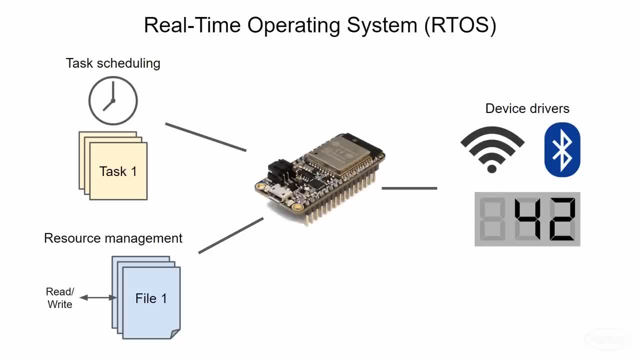 Note that, while most RTOSes provide methods for meeting timing deadlines, that's not the only reason to use an RTOS in your project. The ability to run multiple tasks concurrently can be a lifesaver, as we'll see in a moment. If you've written programs for microcontrollers, including Arduino, you're probably familiar. 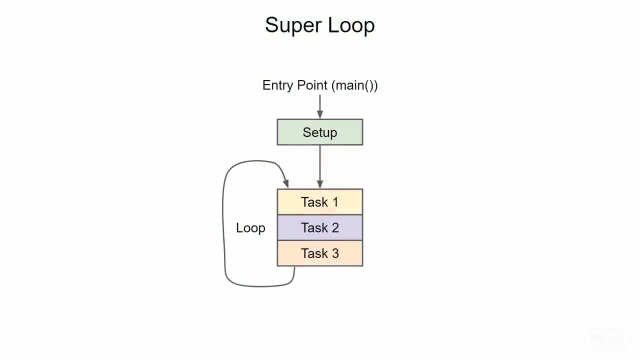 with this kind of structure: When your program starts, it performs some setup functions and then it executes your tasks in a round-robin fashion inside a wildfire a while forever loop. These tasks might read from sensors, perform some calculations based on those readings and then say: display something on a gorgeous. 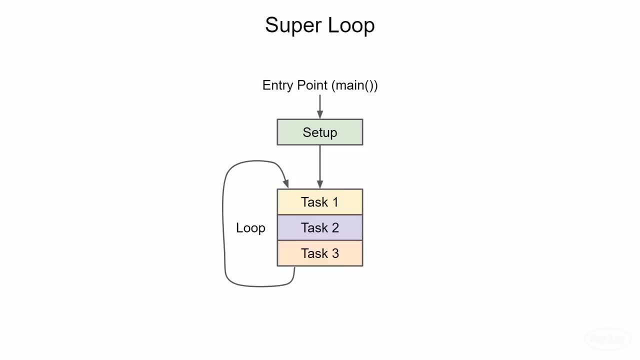 LED display. This type of simple programming architecture is known as a super loop. It's incredibly easy to implement, has very little overhead and is great when you only need to accomplish a handful of tasks on your microcontroller. In fact, there's nothing wrong with the super loop For the vast 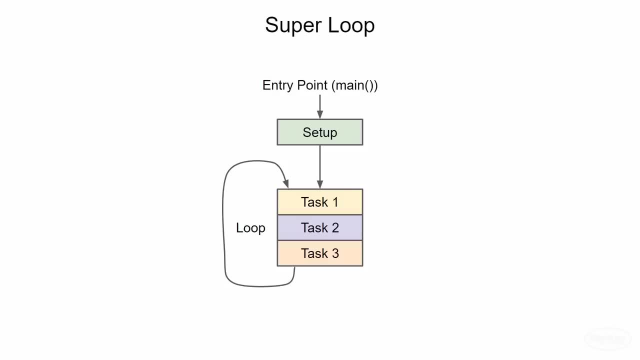 majority of simple microcontroller projects. you're usually better off with this type of program flow as it saves on CPU cycles and memory and it's much easier to debug than using an RTOS. You might even have created a couple of interrupts to break the flow of execution to handle an external event. 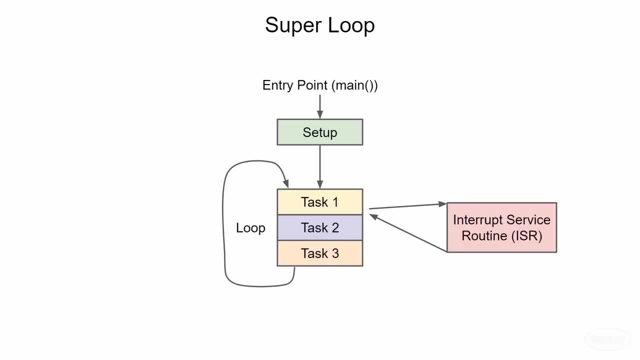 like a button push or perform some action at specific timed intervals. If you need to meet strict timing deadlines for one or two tasks, you might be better off using a super loop, In my experience, if you need to meet a timing deadline of less than about one, 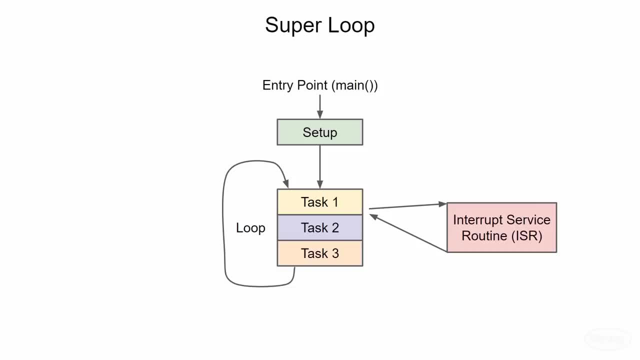 millisecond, your best bet is an interrupt. anyway, If you're trying to do something with an interval of less than a few hundred nanoseconds, you either need an incredibly fast processor or it's time to start looking at custom hardware like an FPGA. Now, the unfortunate thing about this super loop: 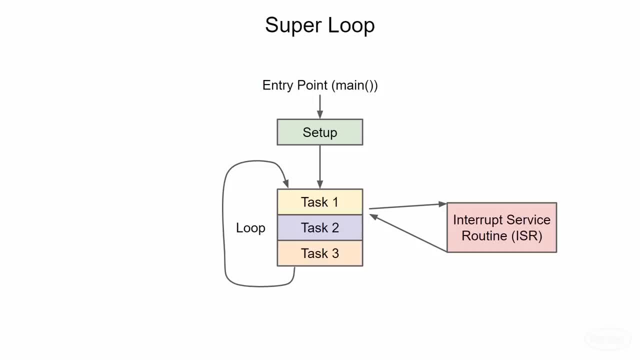 architecture is that you cannot execute tasks concurrently. If task two starts taking a long time and task three is your update display task, you'll start to experience some lag. Similarly, if you're polling for user input, like from a serial terminal or reading a sensor, you 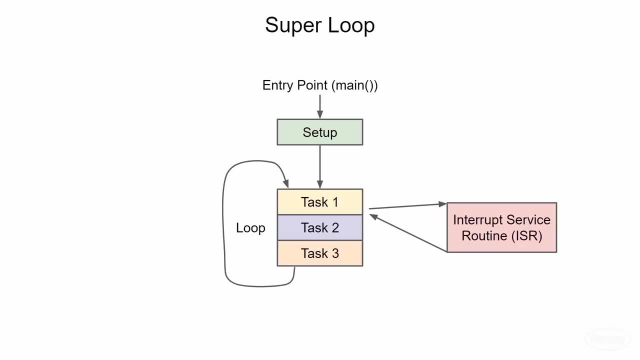 might miss data if other tasks take too long. To fix that, we can use the concept of running multiple tasks at the same time On a multi-core processor. this is actually physically possible. However, since many microcontroller projects are controllers only have one core. the CPU time needs to be split up among the tasks. 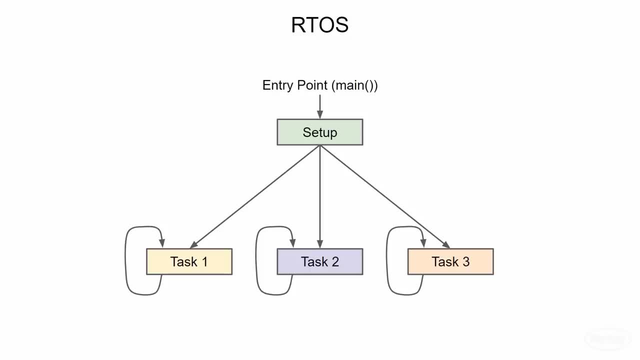 We can also give higher priority to some tasks so that they happen sooner or take more CPU time. For example, if we prioritize the user input task, users will likely experience less lag, but it might mean background tasks take longer to execute. We'll talk more about time slicing and prioritization in a future video. 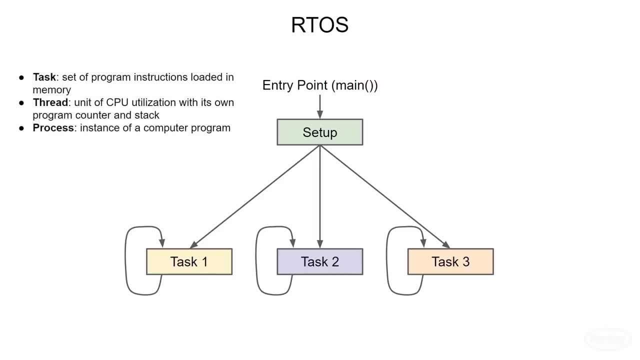 Note the terminology used here. A task is any piece of work we want to get done in code. A thread is a unit of CPU utilization with its own program counter and set of memory. A process is an instance of a computer program that's being executed. 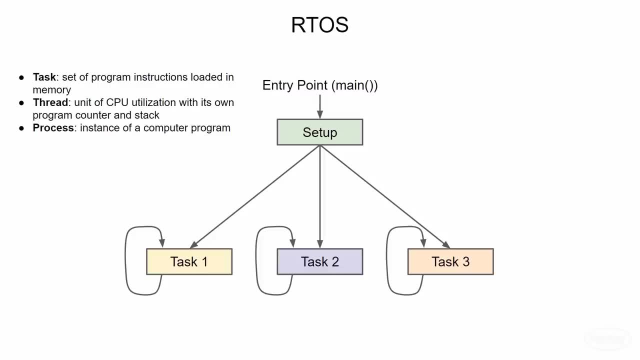 Usually, a process will have one or more threads used to accomplish tasks. Threads within a process will often share resources, like heap memory, and can pass resources to each other. You'll often find that a task is a unit of CPU utilization. An RTOS is capable of handling only one process, but a general-purpose OS can run many processes. 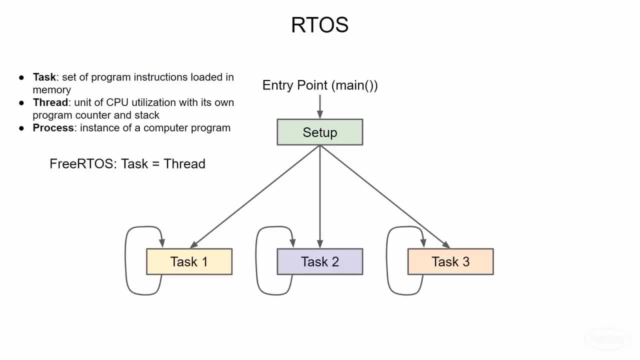 Note that in FreeRTOS, the term task is used to mean something closer to a thread, and you'll often see these terms used interchangeably. Because of this, I will use the term task when referring to units of CPU utilization, so that it makes sense within the FreeRTOS ecosystem. Interrupts still work within an RTOS. So long as they have a higher priority, they will be able to execute tasks. If they have a higher priority than any of the tasks, they will stop code execution for all tasks, run your interrupt service routine and return execution to where it left off. 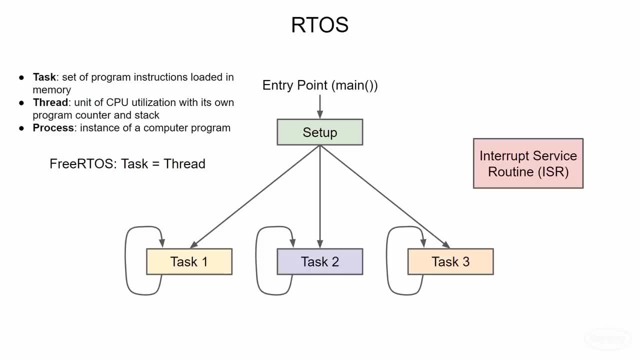 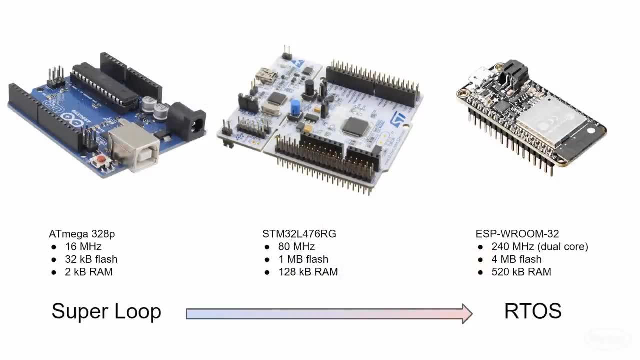 You can have more than one interrupt, but we won't get into handling nested interrupts, which can get nasty. If you're writing code for a simple 8 or 16-bit microcontroller with 2 kilobytes of RAM, you're probably best sticking with the superloop approach and using the inexpensive controller. to do only a handful of tasks. If you're writing code for a simple 8 or 16-bit microcontroller with 2 kilobytes of RAM, you're probably best sticking with the superloop approach and using the inexpensive controller to do only a handful of tasks. If you're writing code for an 8 or 16-bit microcontroller with 2 kilobytes of RAM, you're probably best sticking with the superloop approach and using the inexpensive controller to do only a handful of tasks. Don't cross such a line on your proper C++. 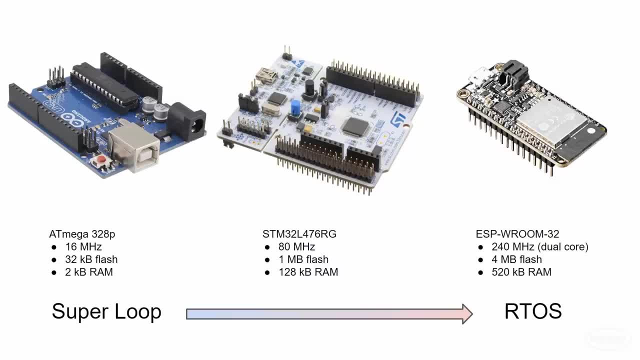 Weiira. Mostly resources are left for the program itself. People have ported FreeRTOS to the Arduino Uno. It's definitely a good way to tinker around with it, but I don't know how useful it is. As you move into more and more powerful microcontrollers, it becomes much more viable for something. 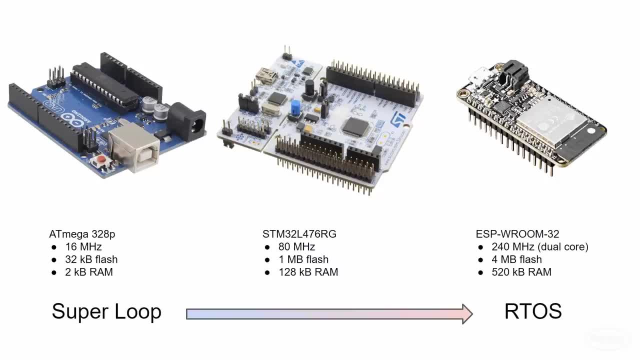 as sparable. Most of your memory and also clock cycles are just for things like a scheduler yourself, someone else's memory- and also clock cycles are just for things like a scheduler metal super loop on something like an ESP32, I usually find that the whole reason I bought. 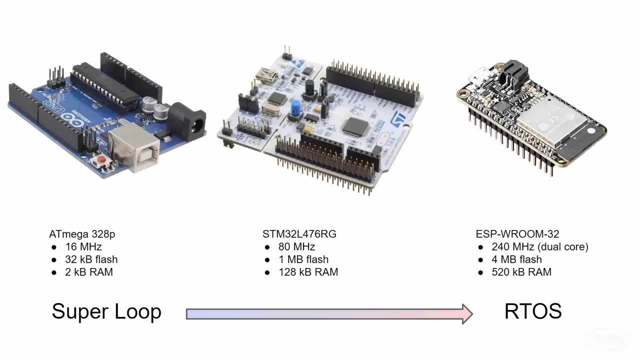 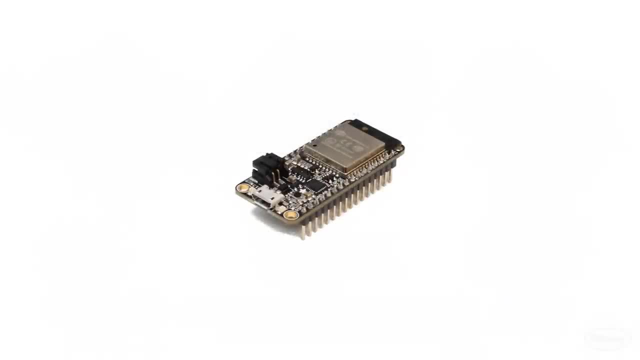 something with that much computing power is to run several concurrent tasks, Which brings me to the ultimate question of why would you want an RTOS? There are a number of reasons, but the best one that comes to mind is for when you need to do several things concurrently. 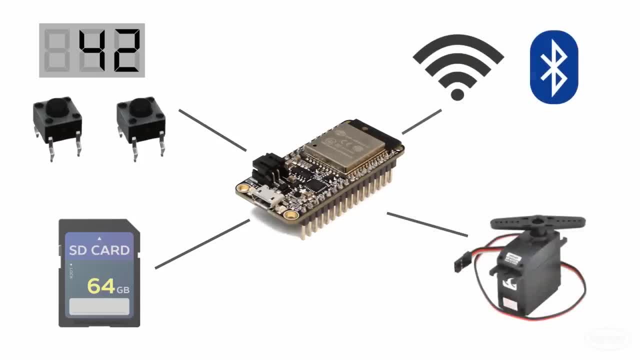 An ESP32 is capable of handling user input, reading and writing to an SD card, controlling hardware and crunching numbers all at the same time. The big one for something like this is the wireless stack. These libraries require large amounts of RAM and processing power. They also need to respond to events from the network in a short amount of time, which means using an RTOS can be a massive help in this case. It can help you divide up these different features into individual tasks. An RTOS can be great if you're part of a team working on a larger project. 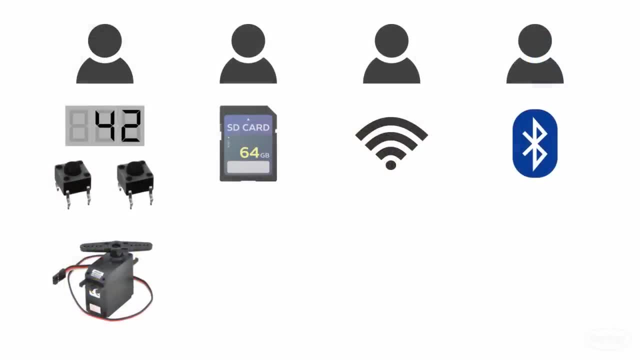 You can divide up the tasks among the team members, knowing that each one will run concurrently. There will be some overhead And debugging to make sure everything works together, though. Over the next few videos I'll go over important RTOS concepts like prioritization and resource. 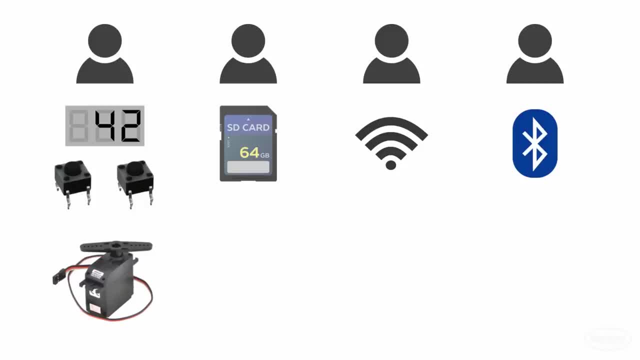 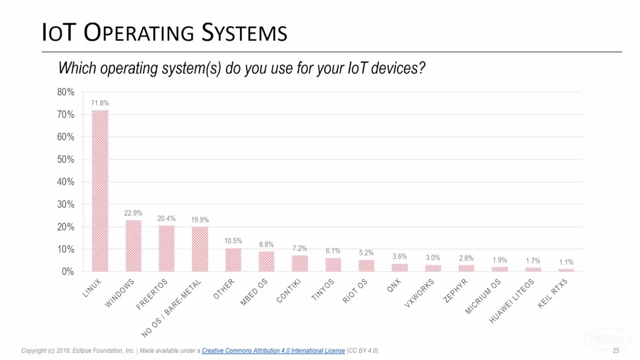 management. We'll practice these concepts by implementing small demo projects in FreeRTOS on the ESP32.. The reason I chose FreeRTOS for this series is because it's currently the most popular real-time operating system for IoT devices, as shown by this 2018 survey from the Eclipse. 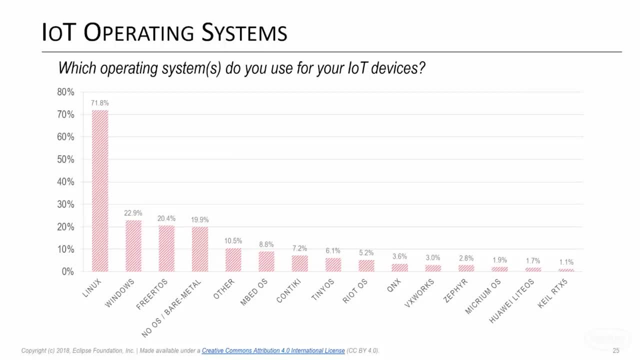 Foundation. While Linux still reigns supreme for most of these devices, It and Windows are general-purpose operating systems. with the exception of RTLinux, You can see that the bare-metal superloop architecture is still quite popular and an acceptable solution to many problems. 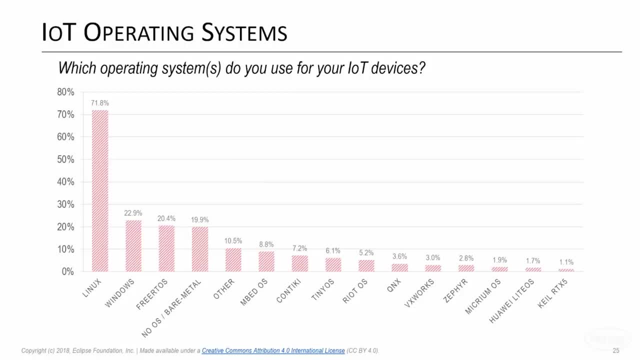 FreeRTOS is also free and open source, making it easy for you to try out. Note that, as of 2017, Amazon has taken over maintenance of the FreeRTOS project. I also recommend keeping an eye on the Zephyr project, as it's a relative newcomer to the 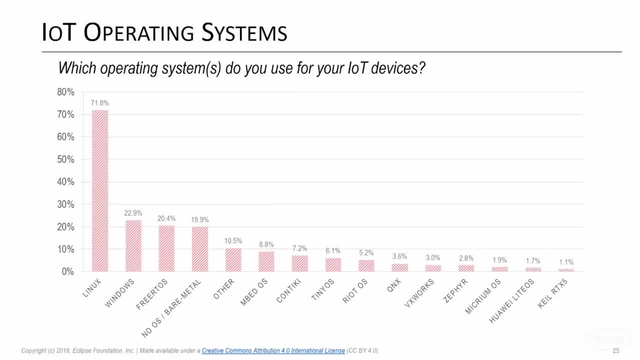 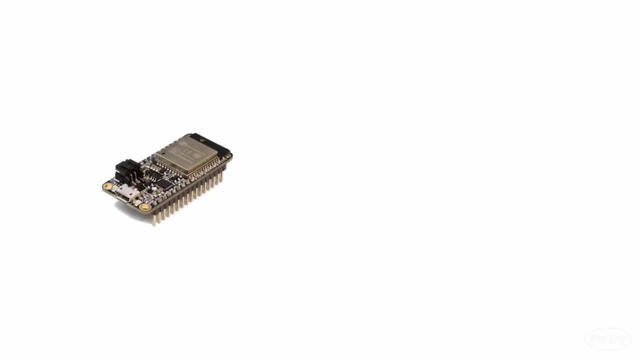 field backed by the Linux Foundation. Thanks for watching. The ESP32 is a powerful IoT microcontroller that's packed with features. Also, you can find inexpensive ESP32 development boards. Any of them should work for this series, as long as they have an associated Arduino package.